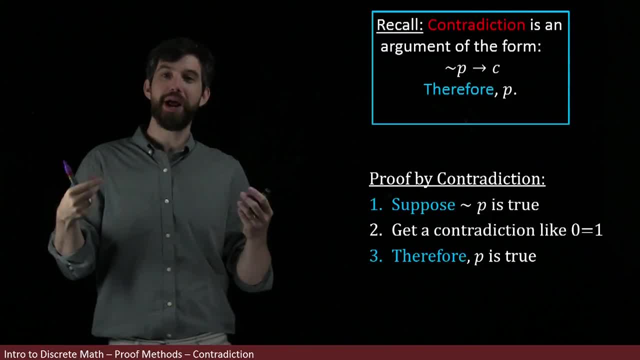 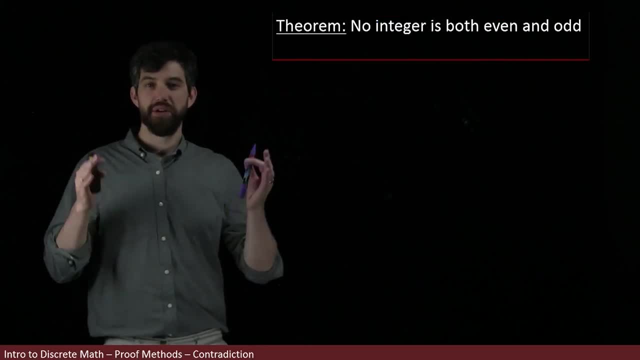 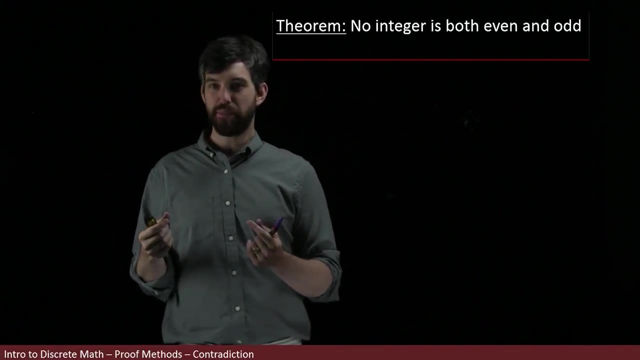 and I'm assuming that statement is false. This is not talking about predicates P of X that depend on a variable. So as an example, let's consider this theorem: No integer is both even and odd. Now the problem here. if I try to prove it directly, 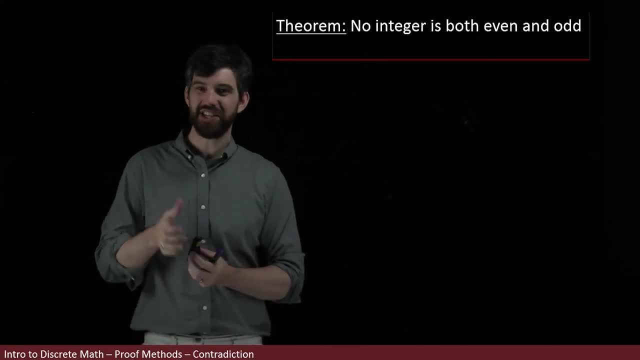 as in: if I wasn't allowed to use contradiction, is that okay? I could check it for one, I could check it for two, I could check it for three, I could check it for four. I could keep on going as long as I hadn't tired. 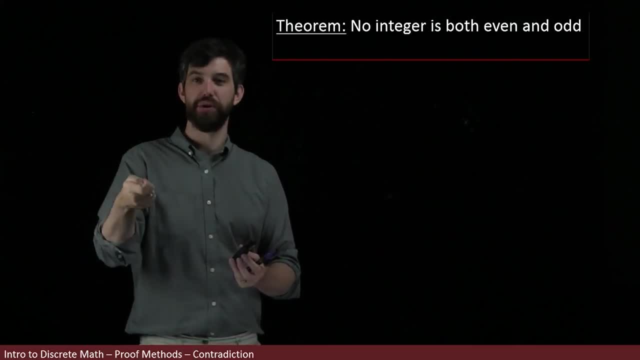 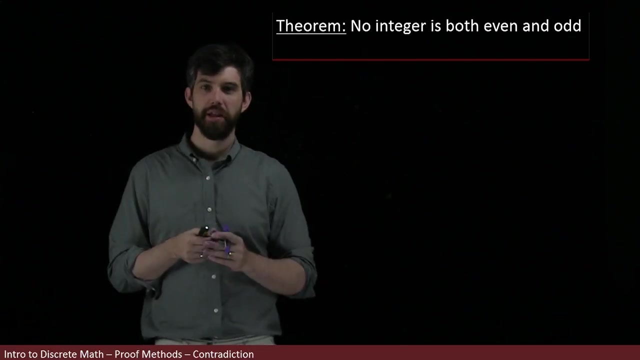 but I hadn't necessarily checked every single integer. Maybe it's somewhere in the billions that you finally find an integer that is both even and odd. But if I'm gonna prove it by contradiction, it's gonna go a little bit faster. Now, before I go into proving this, 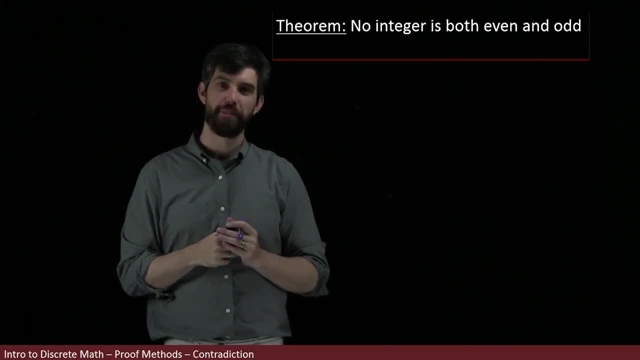 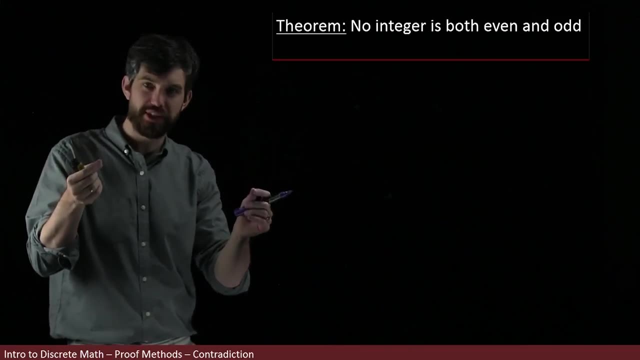 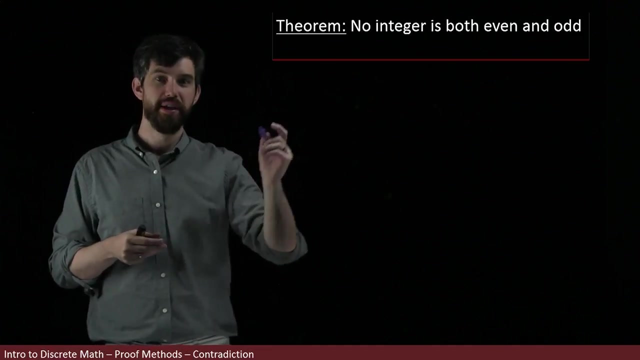 I want to analyze the statement for if logical form When it says: no integer has some property, this is actually a implicit universal statement. This is a claim about every single integer. Every single integer is not both even and odd, So I can rewrite this like this: 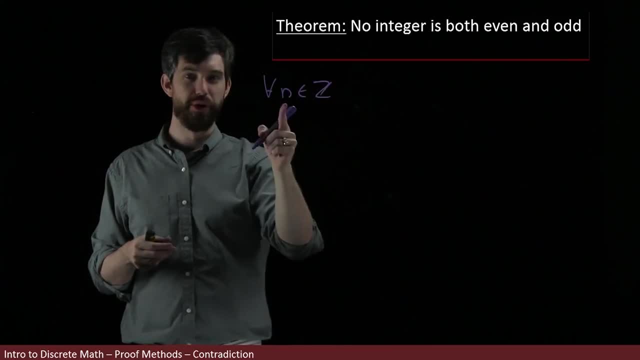 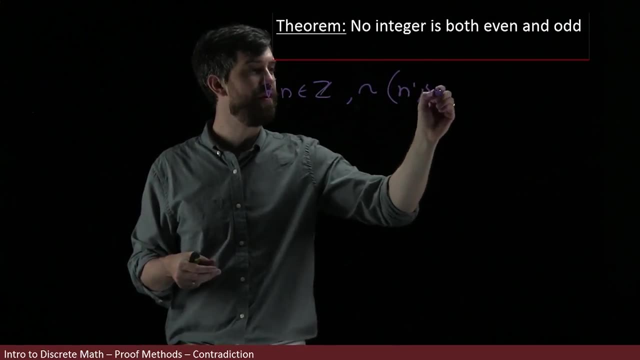 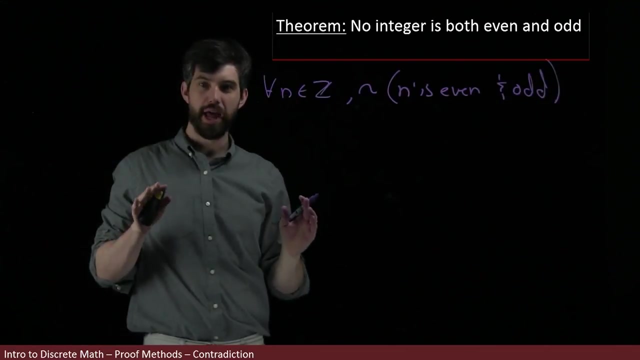 I can say for every integer, in other words, for all n inside of the integers. it is not the case that n is even and odd. I never have both of these different properties. Now, to be clear, this statement was not. 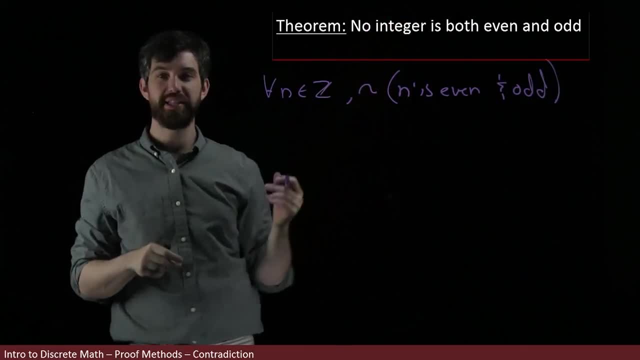 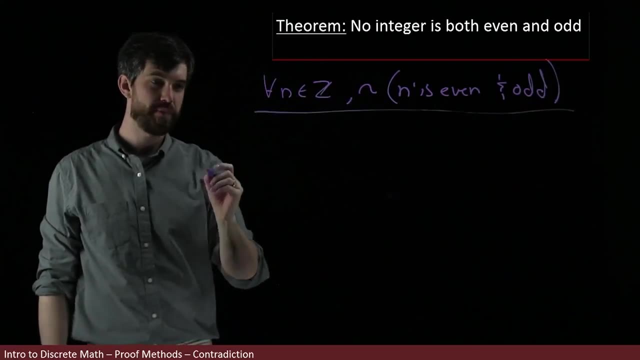 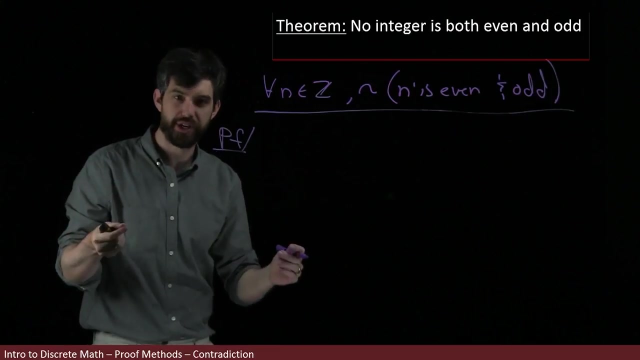 part of my proof. This was just me rewriting my statement and saying that my statement is indeed equivalent to this. So now I'm gonna actually begin my proof. We've decided that what we want to do is prove it by contradiction. So, in other words, I want to begin by assuming. 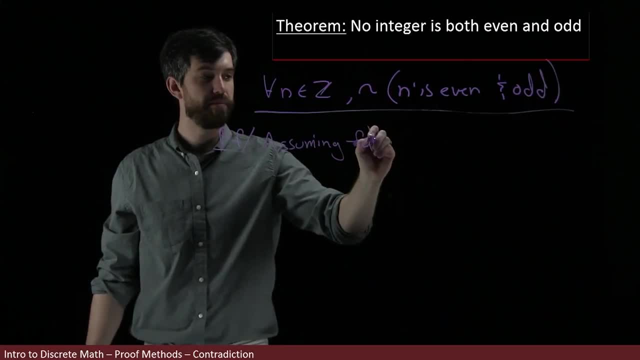 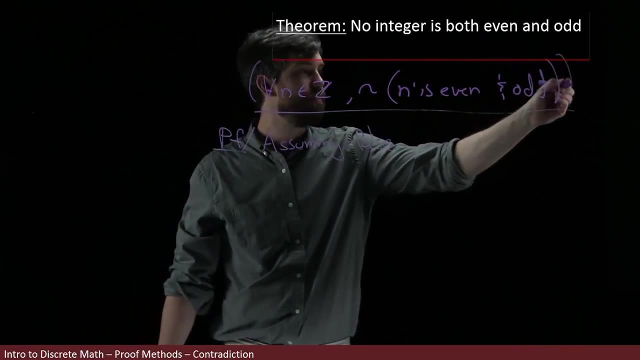 that this is gonna be false And if I'm assuming that it's false, what I'm gonna be doing is thinking that if this is my statement, that I'm gonna be putting a negation in front of it. I'm assuming the negation. 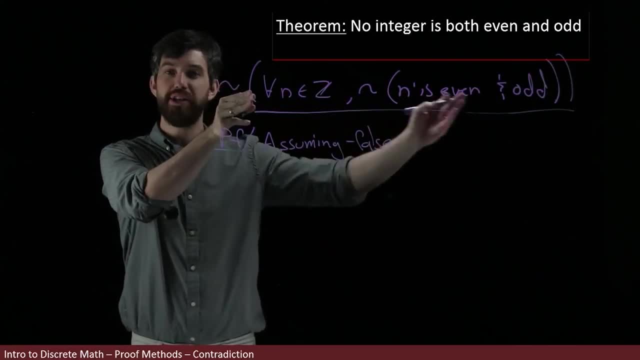 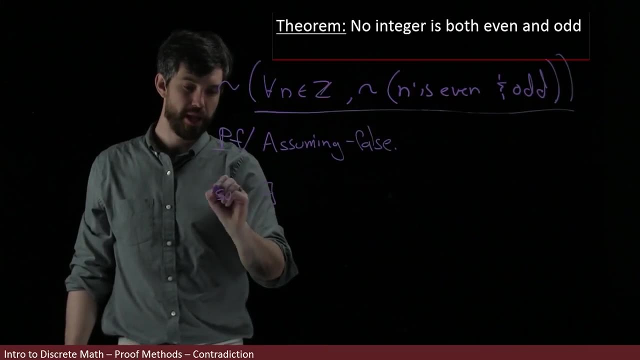 But because this is a quantified statement- and I know how negations work with quantified statements- that what I'm going to get is that for all flips to be in a, there exists. I have an existence of an n inside of the integers. 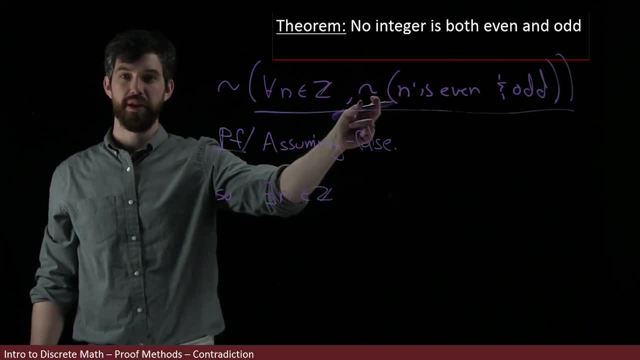 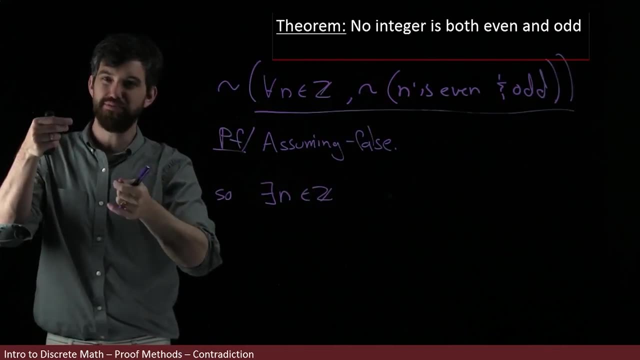 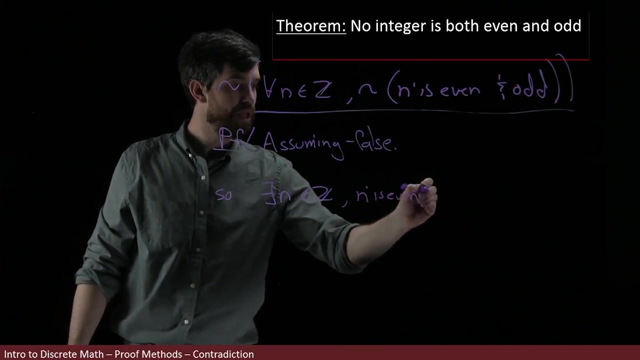 And then the negation moves inside. But notice how we already have a negation moved inside. So if I take this negation and move it inside, I have two negations and a double negative cancels. So what I'm just left with is n is even and n is odd. 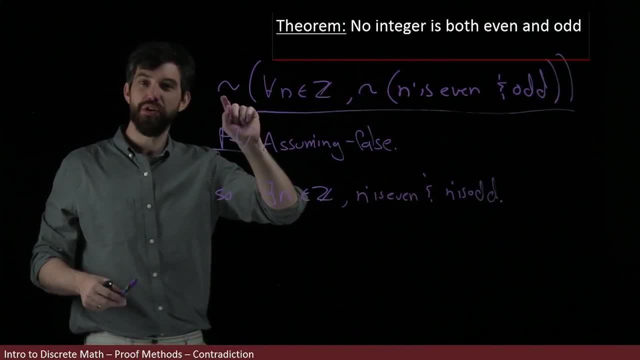 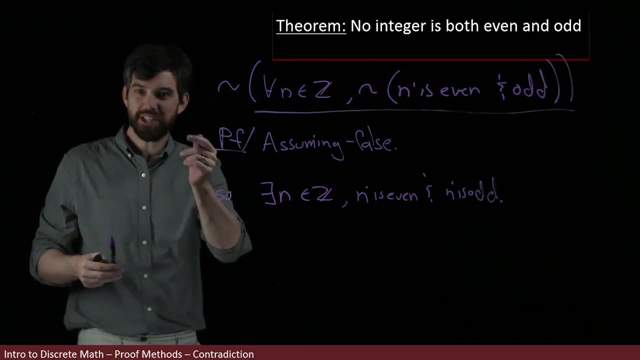 So the way to think about this is: if my original statement is no integer is both even and odd, then if I'm gonna assume that that thing is false, it says: well, there has to be at least one that is both even and odd. 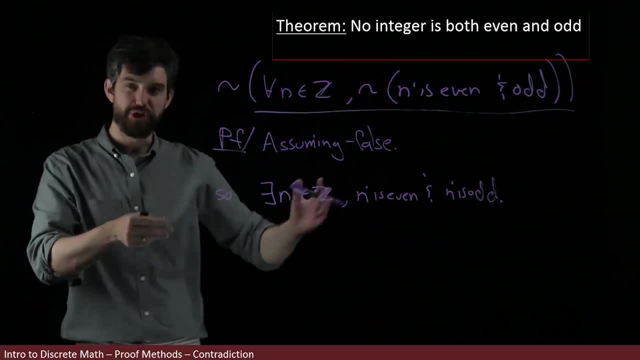 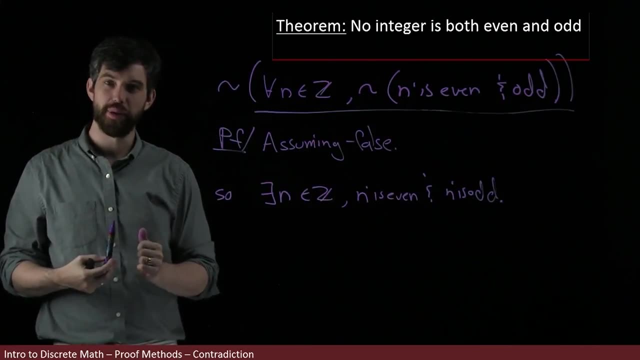 And that's my claim here. Okay, so I've got this assumption, and what's the next step? in most of our proofs, Let's apply the definition. I'm claiming this is even and I'm claiming this is odd. But what does that mean? 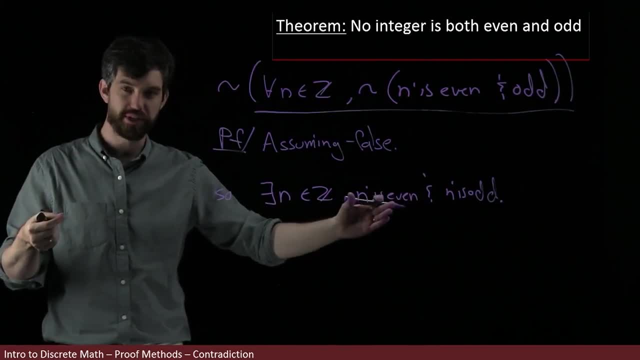 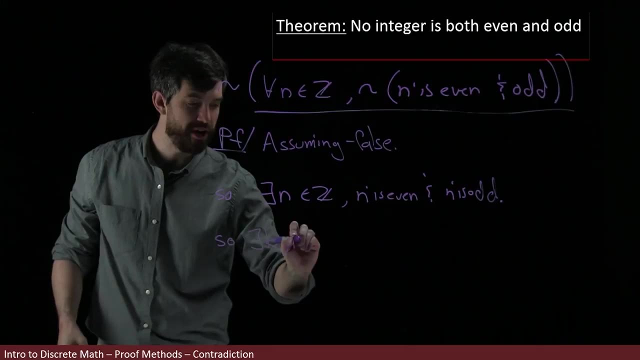 Well, it means that there exists two other integers, so that I can write it in the following way: So there exists a- I'll call them K1 and K2, because I need one for the even and one for the odd. These are both gonna be integers. 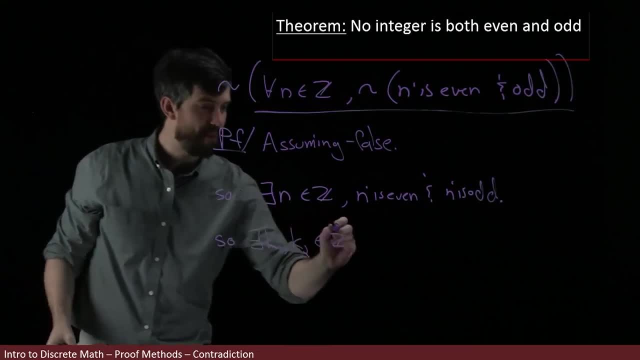 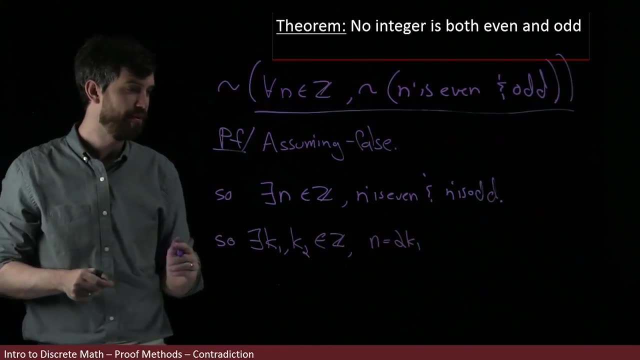 And they have the property that I can rewrite the n and the m. I can say that my n is gonna be twice the K1, because it's even that's what it meant to be, even that you can write it as twice something. 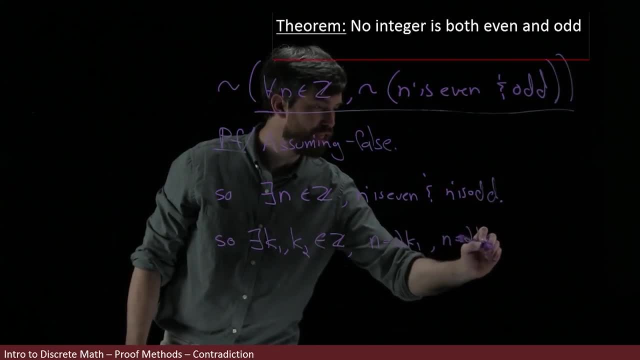 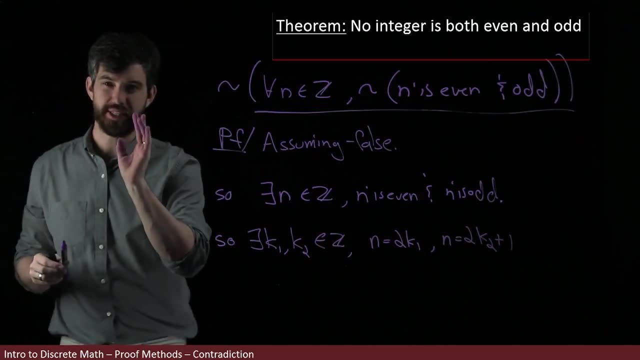 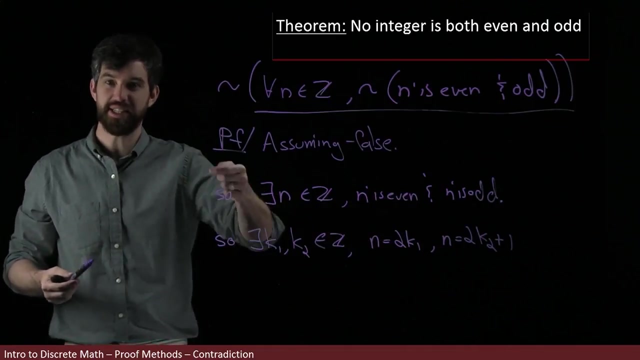 And that the n is gonna be 2K2 plus one. By the way, it's very important here that you don't use the same K. This is often a place that people can make mistakes in their proofs, Like the claim for n is even is there exists a K. 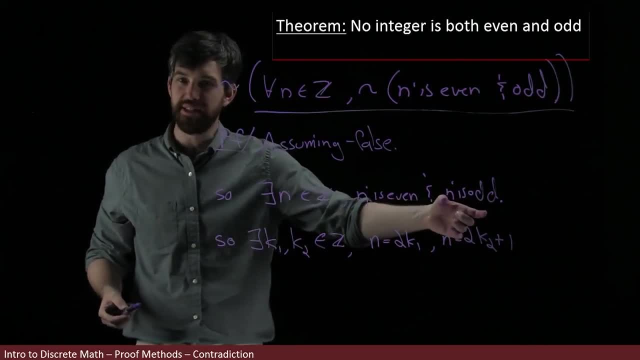 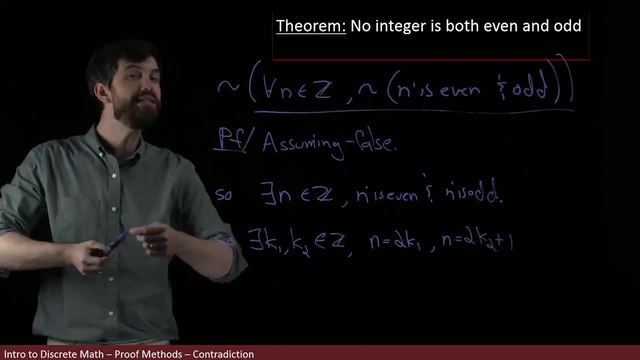 so it can be written as 2K. And the claim for n is odd is there exists a K, so it can be written as 2K plus one. But because I'm doing both of these at the same time, they don't necessarily have the same K. 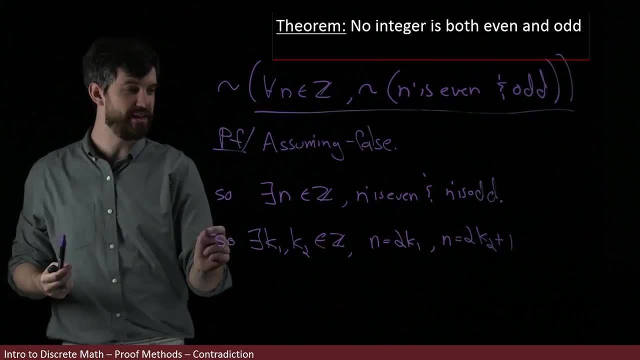 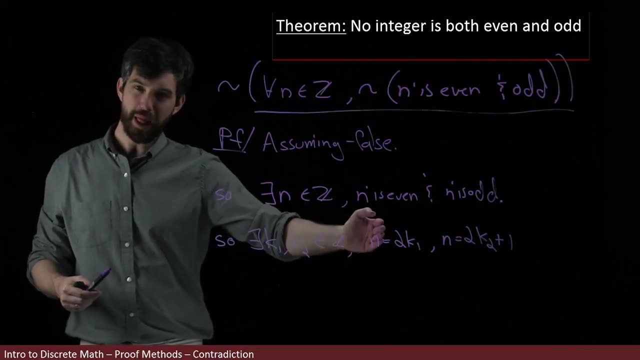 So I choose different ones, I index them as K1 and K2, and I get these two different claims All right. so there was my assumption, was the first two lines. Now I've applied my definitions. Now I'm gonna apply my definitions. 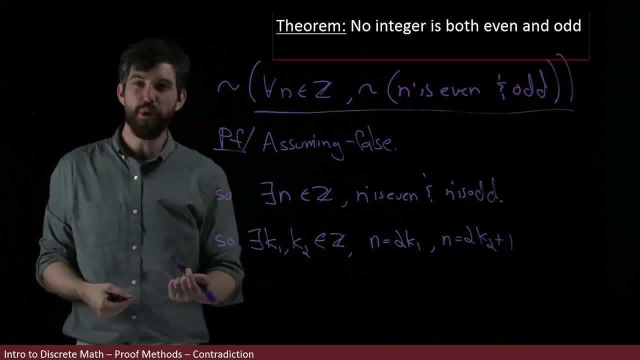 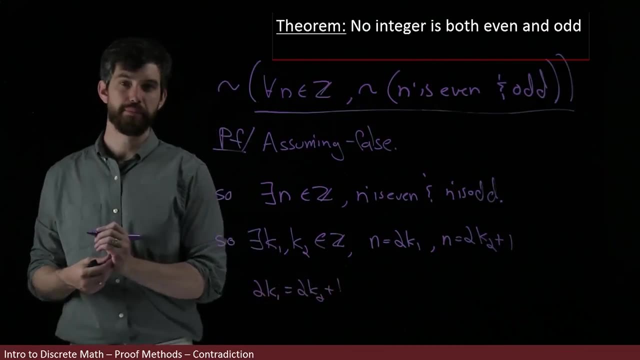 Now I'm gonna apply my definitions, And what do I get here? These are both n, so I'll set them equal to each other. So 2K1 is equal to 2K2 plus one. And then moving the K2 to the other side. 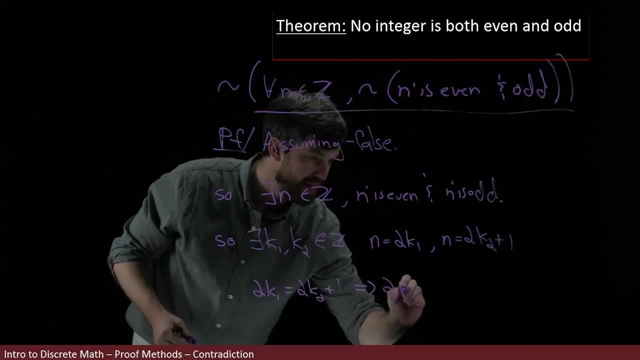 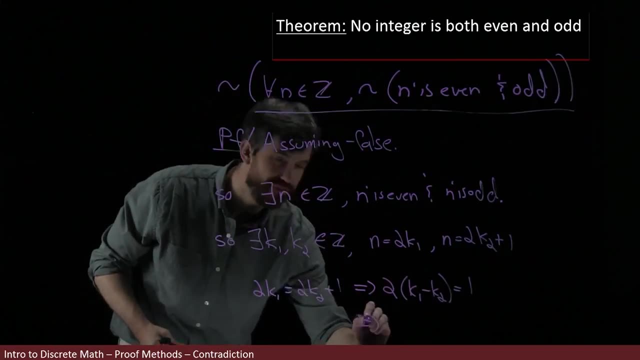 and pulling out the two, I get the formula twice: K1 minus K2 is equal to one. And finally I'm gonna divide out by two. I'll show you why in a moment I can divide out by two to get that. 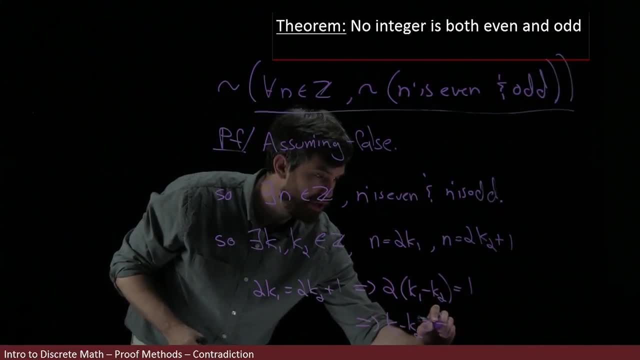 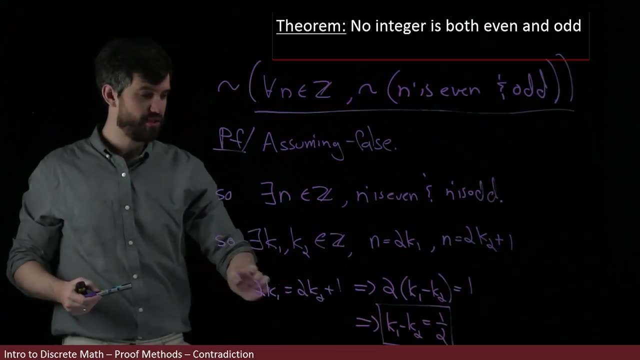 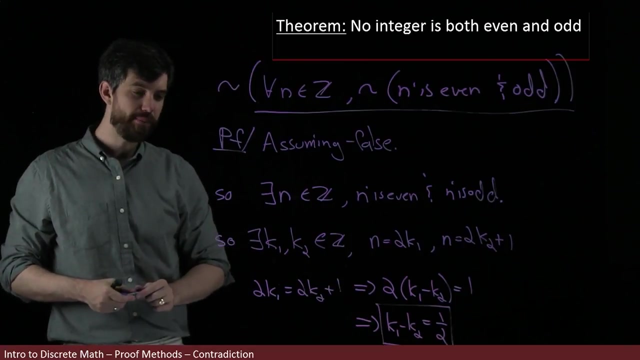 this difference, K1 minus K2, is equal to one half. Now I claim that this result- that K1 plus K2 is equal to half- is gonna give me a contradiction. So why is that the case? Well, if I look at my K1 and my K2,. 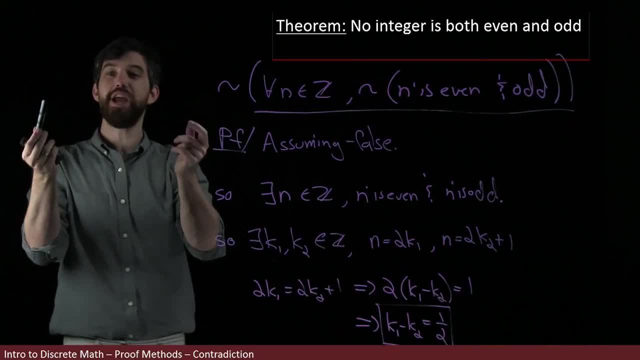 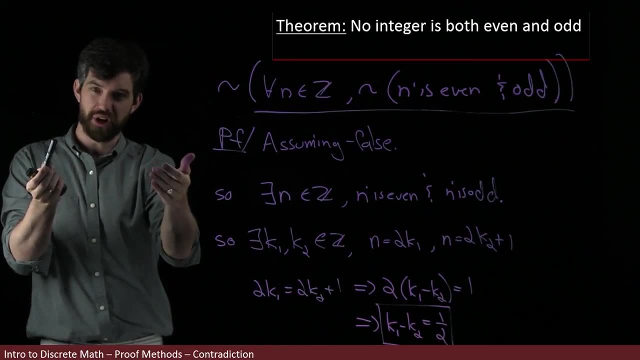 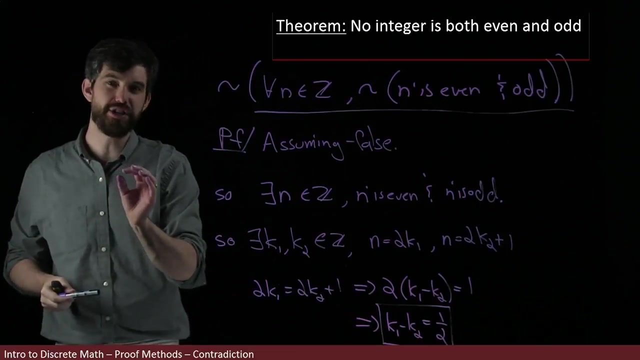 here they were. they were both integers, So I've assumed K1 and K2 are integers And then the difference of two integers is likewise an integer. So K1 minus K2 is gonna be an integer. But I just showed you that K1 minus K2 is not an integer. 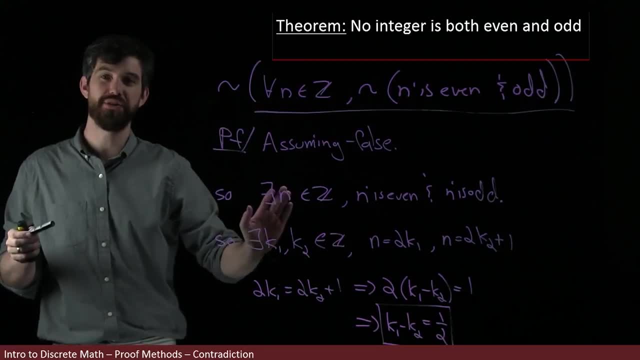 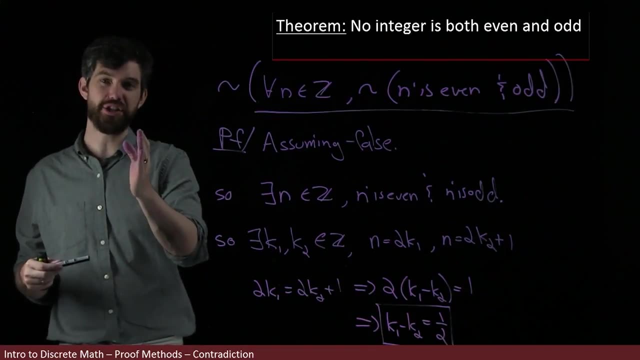 It's a fraction, It is one half, It is a rational number. that is not an integer. So I've got two different claims that are contradictory. I've got the claim K1 minus K2 is an integer. I've got the claim K1 minus K2. 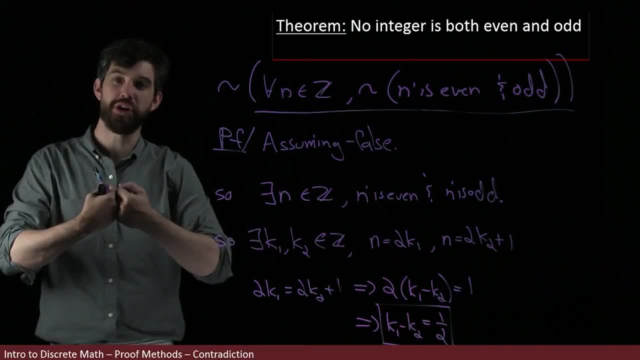 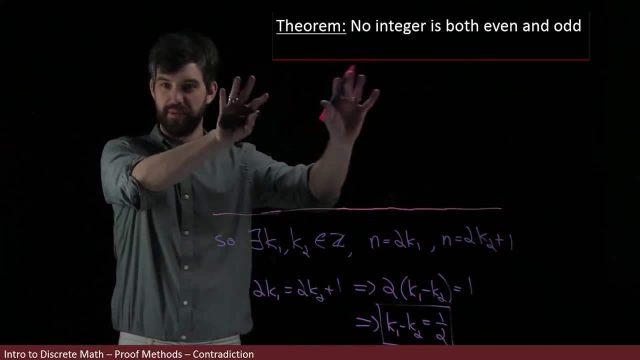 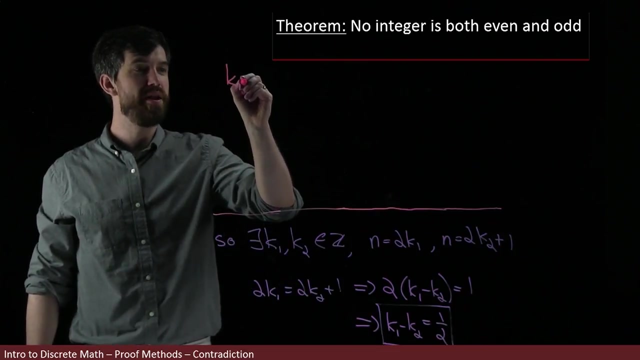 is equal to this fraction one half. That contradiction cannot be So. clearing up some space for myself. what I have is this contradictory claim: first, that the K1 minus the K2, that this is going to be an integer which we got from noticing that it was the difference. 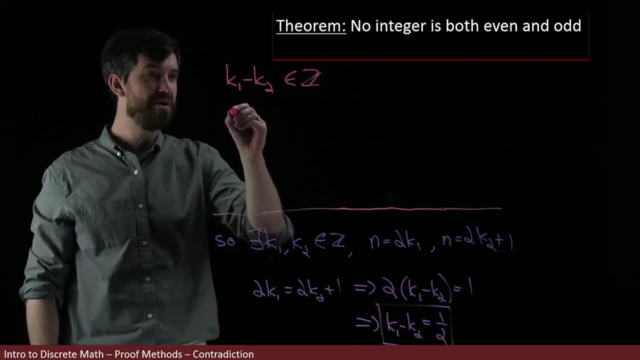 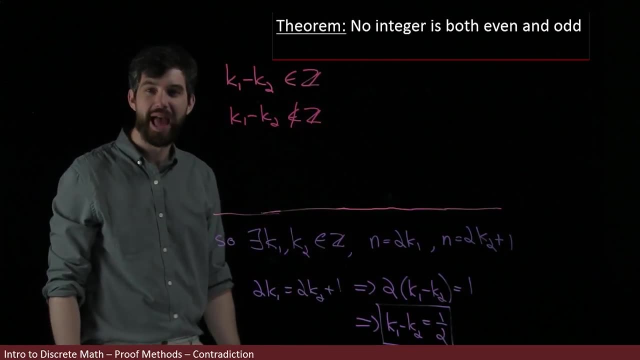 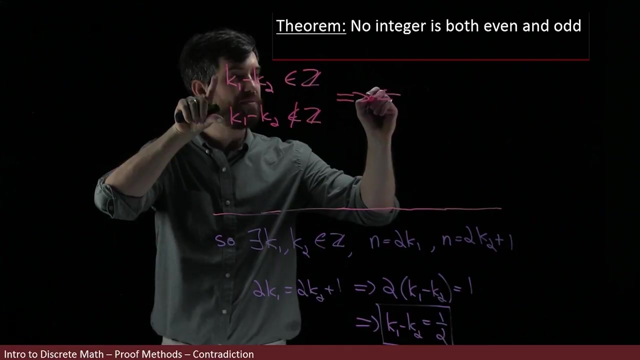 of two different integers And then, from what I have down here, I've got that my K1 minus K2 is not an integer because it's equal to a half and a half is not an integer, And this is a contradiction- The symbol I sometimes use for contradiction. 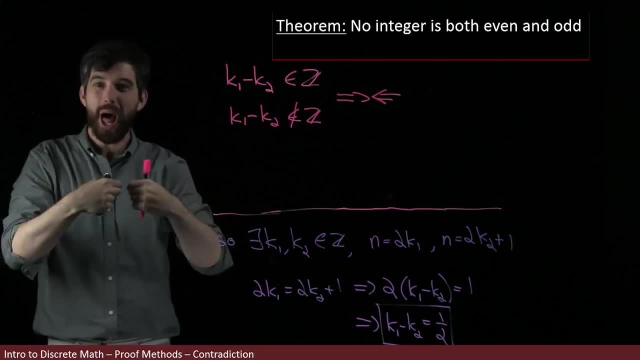 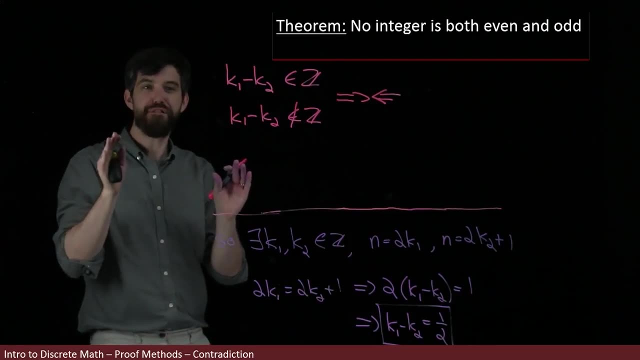 is two arrows that are both pointing to each other because they, like, imply nothing. But either way, what I mean by this is a contradiction. Okay, so how do I finish off the proof here? I began with the assumption that there was an even integer.